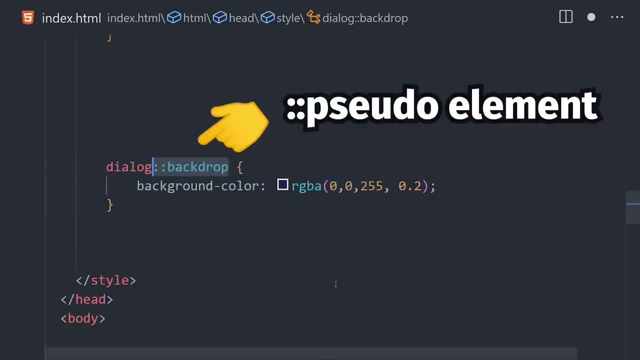 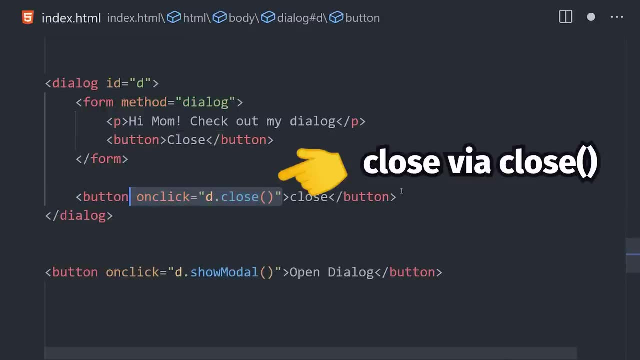 with a backdrop, The backdrop itself has its own pseudo-element that can be styled with CSS. We can then close the modal by either submitting a form inside of it with a method of dialog, or by calling its close method on some other event. This makes life so much easier because 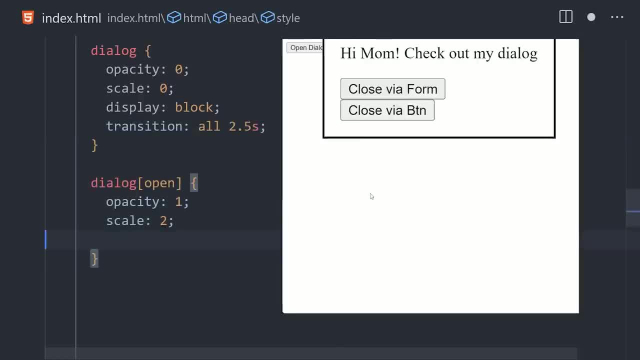 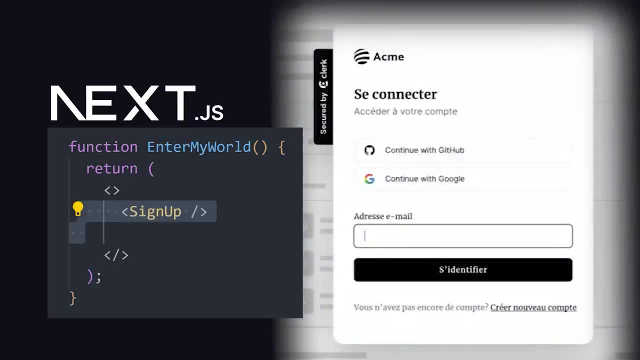 you can animate it using simple CSS transitions. And speaking of making your life easier, today's sponsor is Clerk, who provides the most beautiful user authentication solution I've ever seen. By dropping a few components into your favorite full-stack framework, you get a professional. 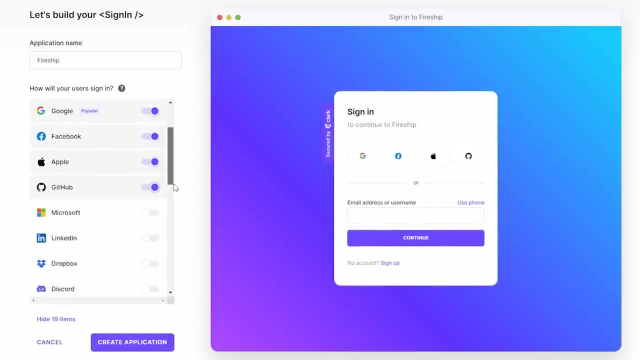 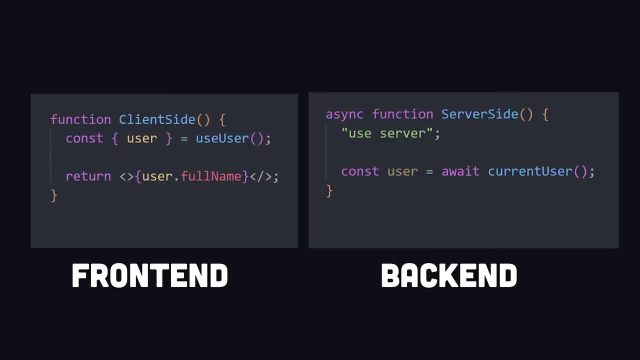 UI that can handle a variety of different sign-in methods, like passwords, magic links, social sign-on and multi-factor auth. Once signed in, developers can easily access the current user from both front-end and back-end environments. In addition, Clerk provides the 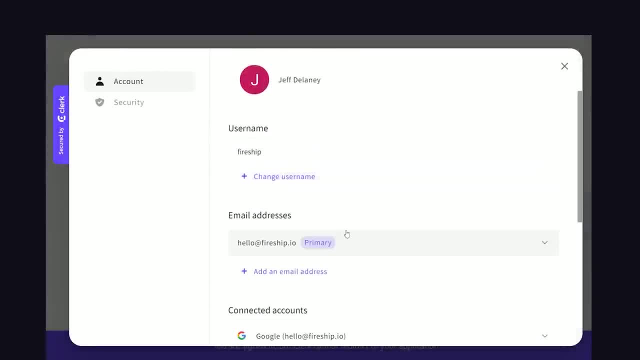 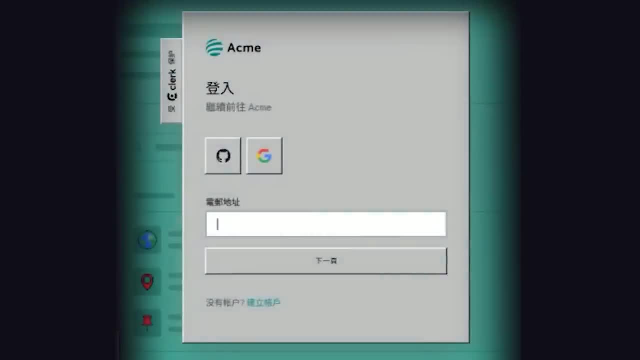 UI for users to customize their own data and handles advanced security requirements like session management per device- features that could take weeks to roll out on your own- And the UI is fully customizable. I had a lot of fun switching from retro to neo-brutalism- These. 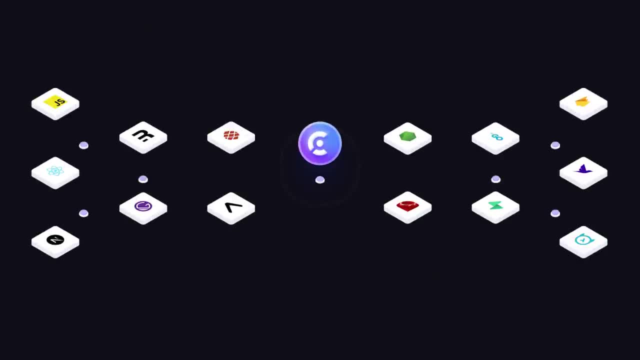 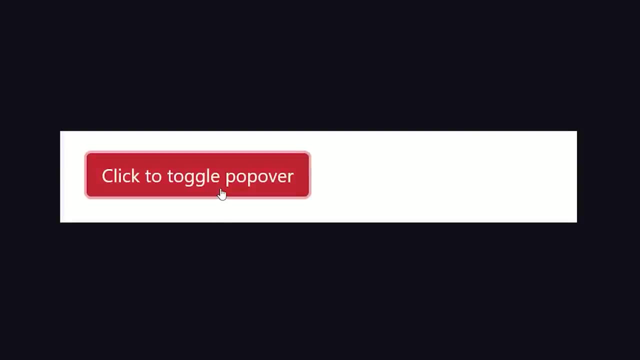 components can be dropped into any React framework and play well with popular back-ends like Firebase, And it has a free tier up to 5,000 users. Give it a try with the link below. Native modal windows are great, but another feature that's annoying to implement is the 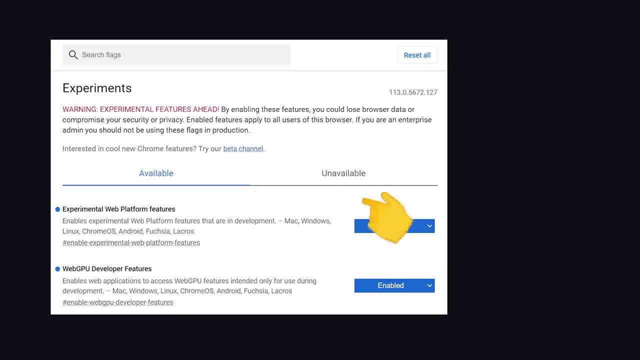 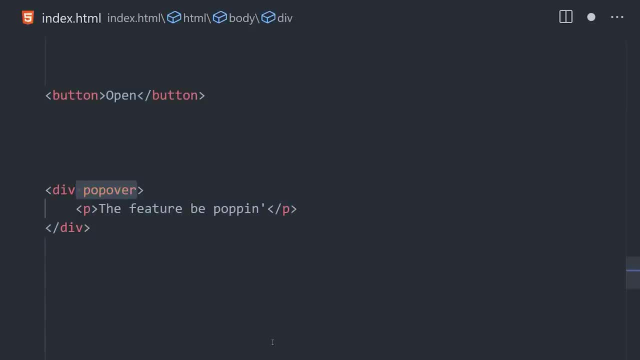 popover. Luckily, native popovers are also coming to the web As of today. this feature is experimental, so you'll need to enable it with a flag, but basically it provides a couple of attributes like popover, target and popover, which allows you to show and hide content without the 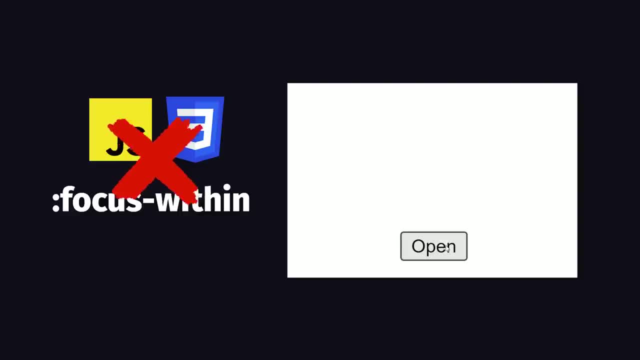 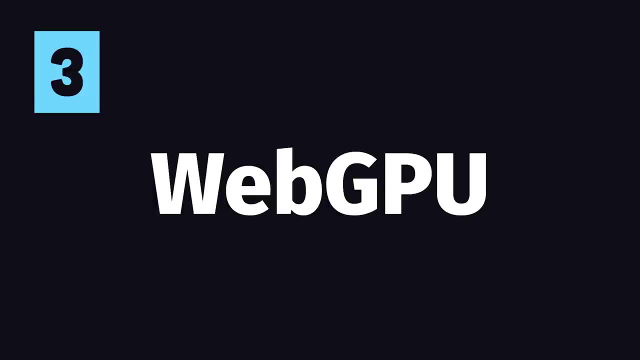 need to write any JavaScript or tricky CSS that uses focus within. Just match the element ID to the popover target and you're done. That'll be a nice quality of life improvement and you'll be able to use it in a lot of different ways. But the next feature, WebGPU, is easily the most 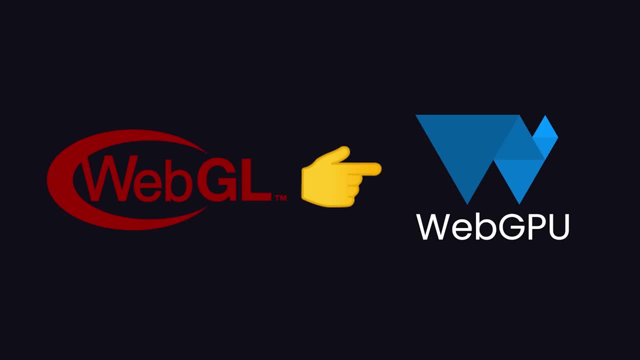 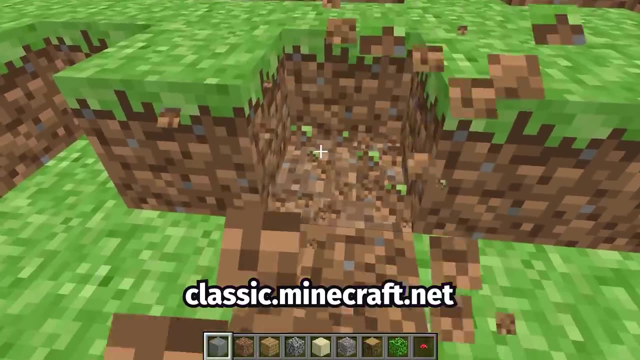 important feature on this list, even if you never use it. It's basically the successor to WebGL, allowing browsers and web applications to take advantage of GPUs. It is under an experimental flag today, but many libraries, like Babylonjs, fully support it already and support for 3.js. 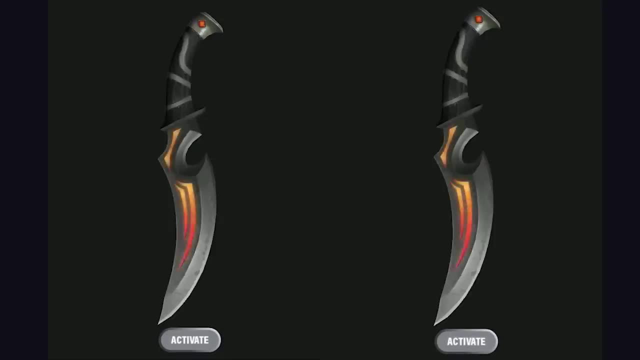 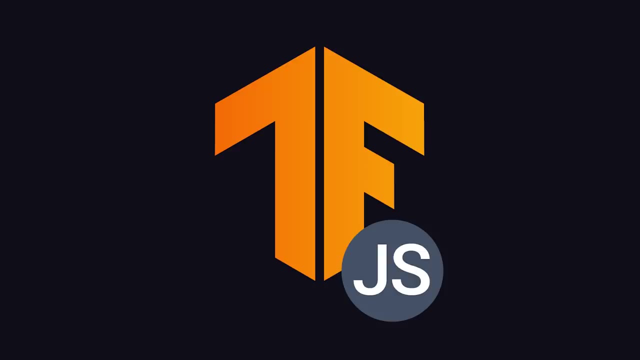 is underway, And that means 3D graphics and games are about to get way faster on the web. I'm using it right now with Babylonjs and, as you can see, the WebGPU version is far more majestic. And not just that, but libraries like TensorFlowjs support it, which means that you can use it to. 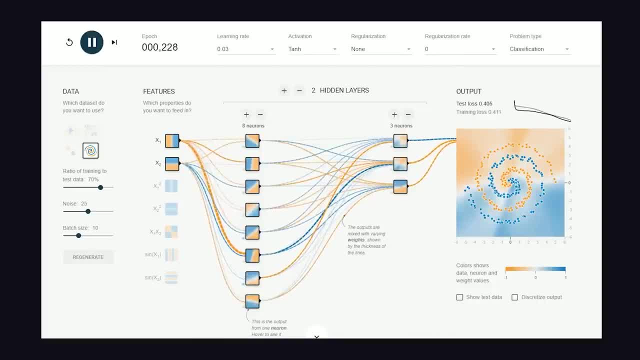 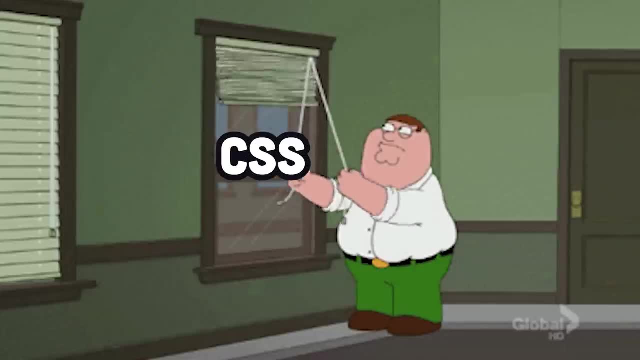 build web apps where end users can train machine learning models without the need to download a bunch of Python libraries or use a notebook in the cloud. That's pretty cool, but for most web developers, the biggest challenge is writing good CSS. Next on the list we have container queries. 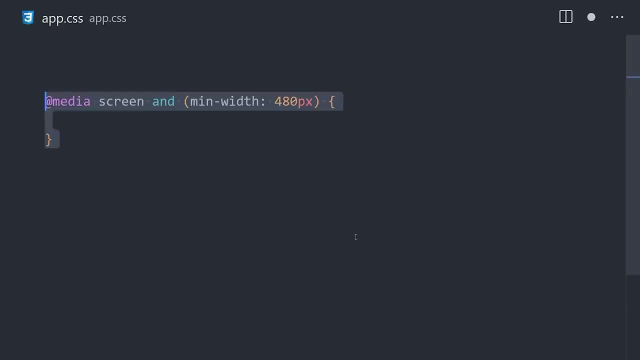 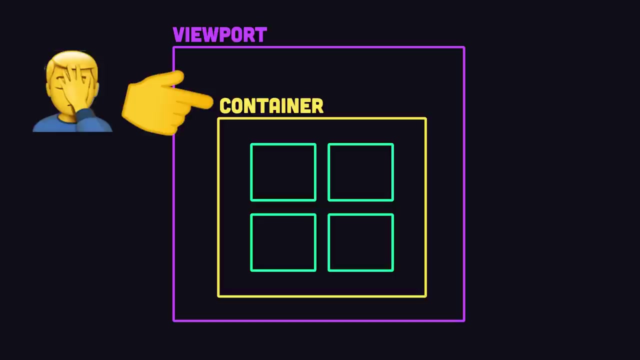 To build responsive websites. developers often use media queries where you apply different styles to an element based on the size of the viewport. The problem is that in many cases, you're not worried about the viewport, but you're worried about the parent container of an element, And 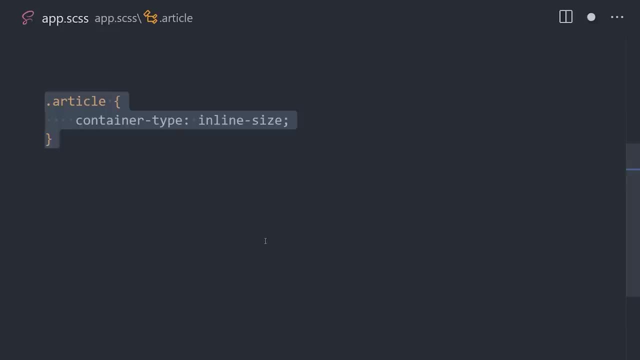 that's always been really hard to deal with until now. With container queries, you first create a containment context with a container-type property. Then from there you can use the container-at rule, which can apply different styles based on the nearest ancestor container. 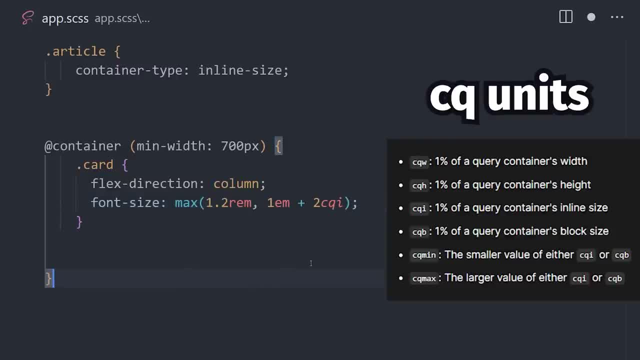 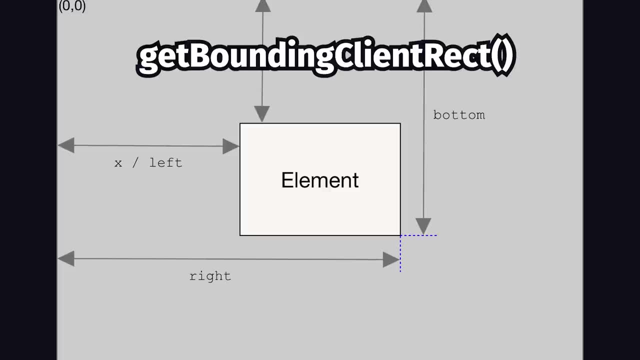 In addition, there are a bunch of new units like container query width and height that allow you to compute the proper size of the children directly in the CSS. In the past you might run into situations where you have to actually get the bounding box from JavaScript then solve some. 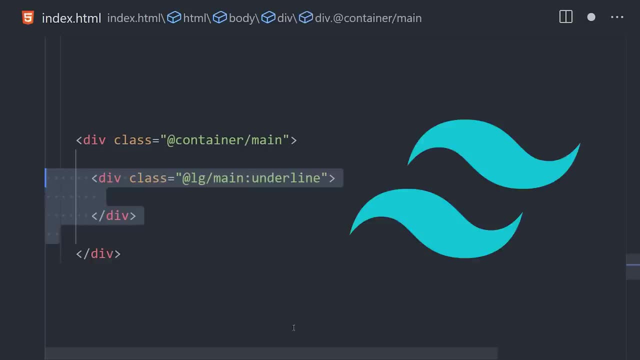 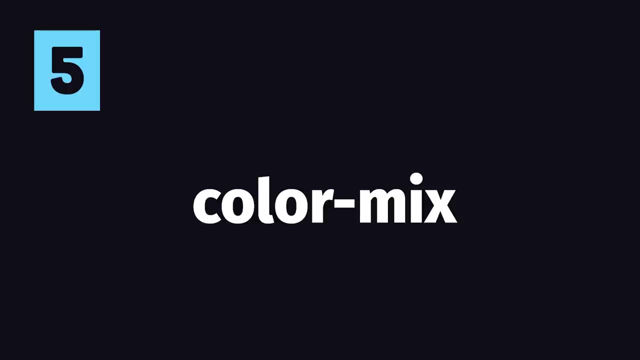 crazy differential equations to get the div in the right place, And you'll be happy to know that there's an official Tailwind container queries package that allows you to declare these containers in your HTML. Another cool CSS feature you might not know about is color mix. I've used tools like 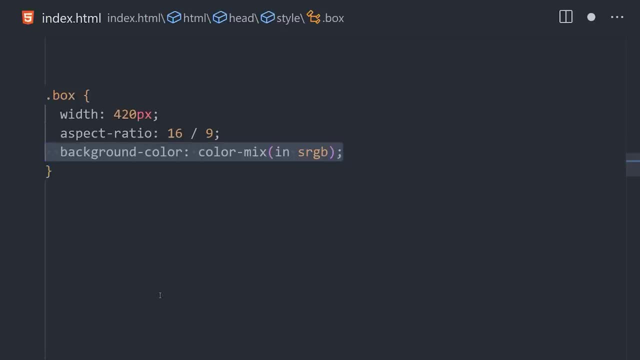 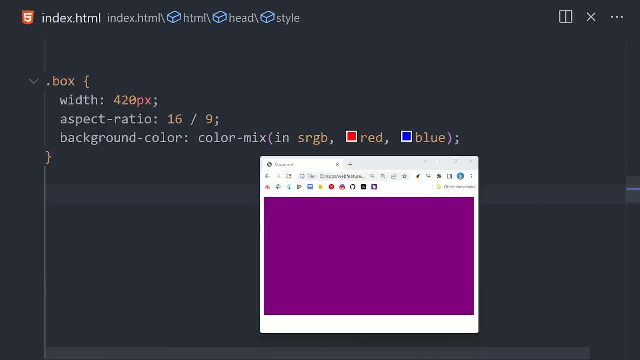 Sass to mix colors in the past, but now we can do it natively in CSS. It's a function that takes two color arguments and mixes them in a specified color space, Like in this example. if we mix red and blue in an RGB color space, we get purple as a result. That's not very useful on its own, but it 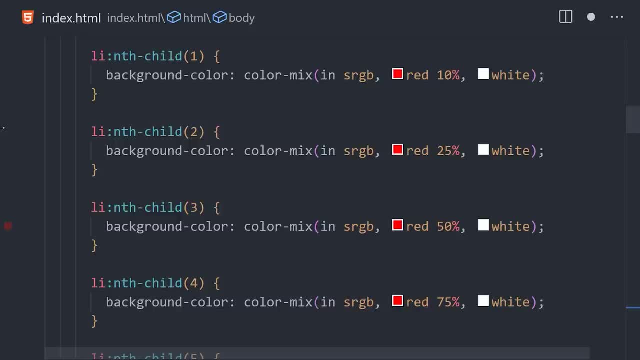 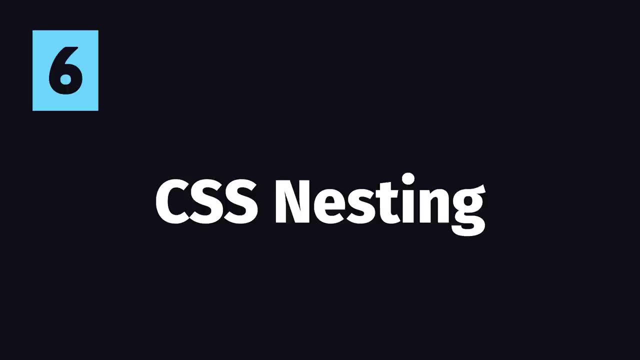 makes it easier to do effects like this, where I have a list of items that mix red and white together to create a gradient effect that occurs over multiple elements. But speaking of features from Sass, another huge one is CSS Sass nesting. I can't believe it's taken this long, but it's almost fully supported in all modern 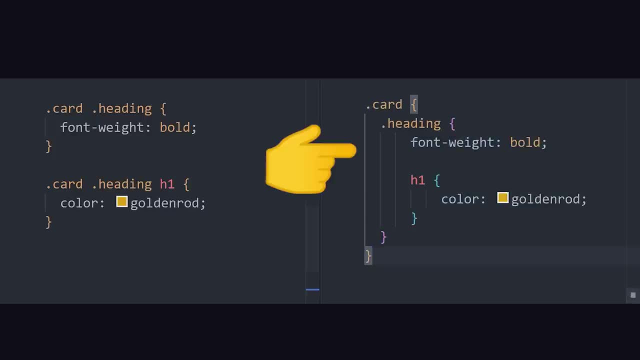 browsers. It's purely an ergonomic feature that allows you to write styles in a far more concise and readable way by nesting them inside a parent, just like a kangaroo in a pouch, which eliminates tons of duplicated class names from your code. But another very interesting new feature is color. 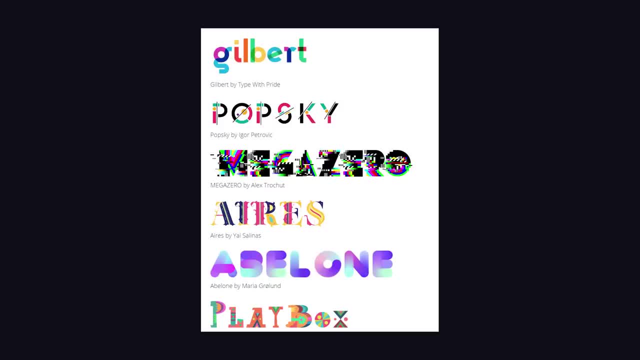 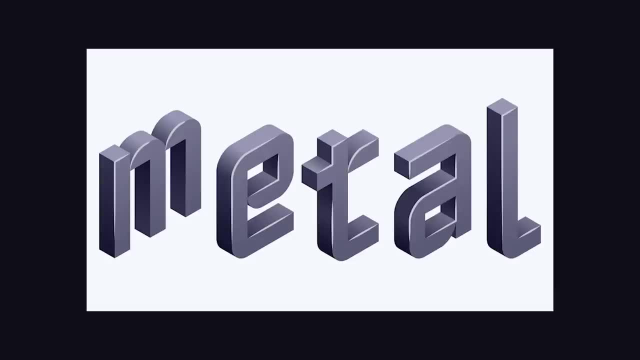 fonts, also known as chromatic fonts, that use multiple colors inside of a single glyph. This opens up a whole new world of possibilities, because now you can customize the entire color palette of a font and create some crazy effects like 3D gradients. 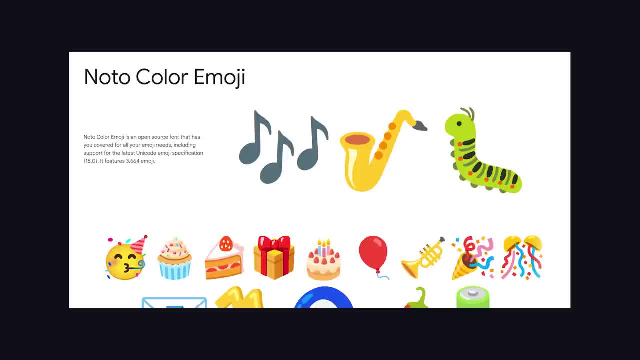 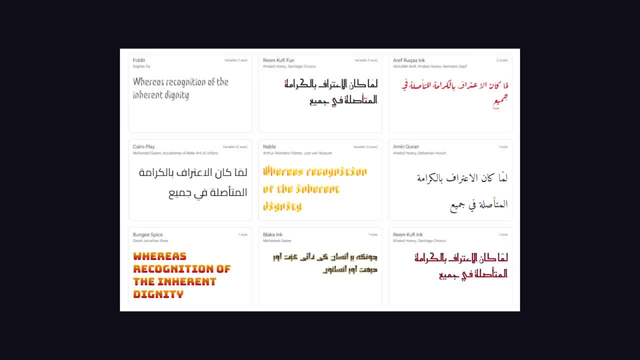 What's cool about this is that they're still interpreted as regular fonts in the browser, whereas previously, stuff like this would only be possible with your own custom vector graphics. There are only a few color fonts at the moment, but it will be interesting to see what else comes out in the future. 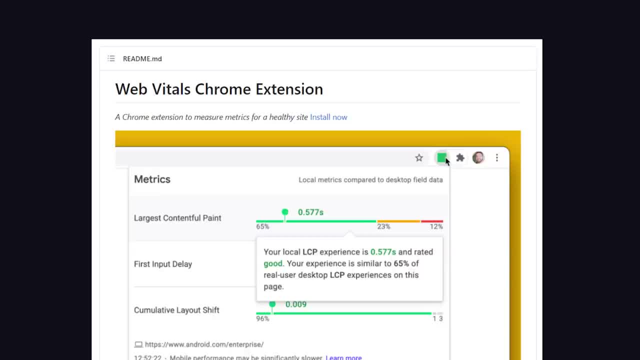 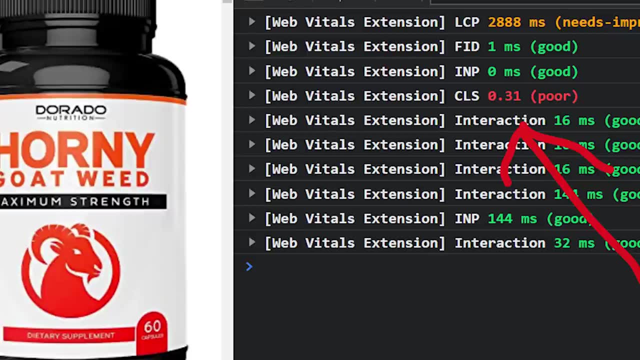 But the next thing I want to look at is performance and the new Web Vitals plugin for Chrome. You can measure the performance of any website by running a Lighthouse report, but the process is kind of slow and cumbersome. This plugin will console-log performance metrics as you use a website and it can pinpoint performance issues like layout shift. 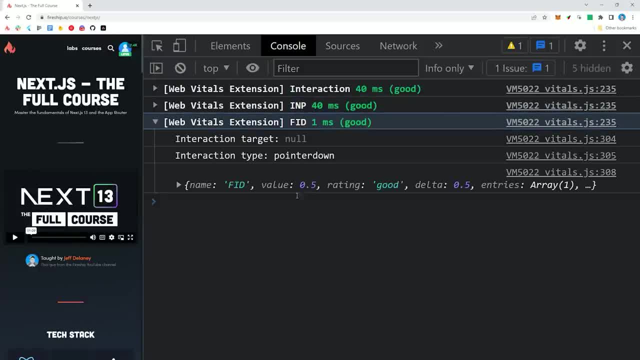 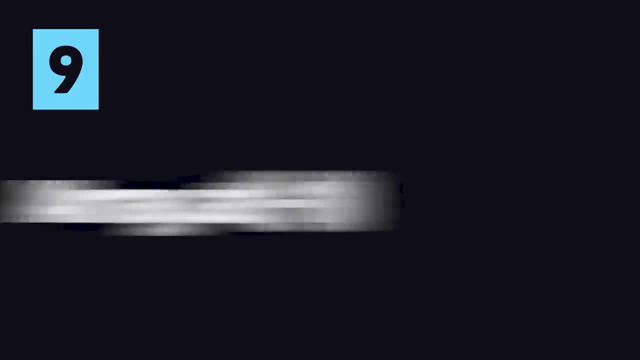 and point you to the exact element that's causing the problem. There's a ton of things to consider when it comes to performance, and I have a full video on that topic on my second channel if you want to learn more. But now it's time to talk about some new JavaScript features like array at 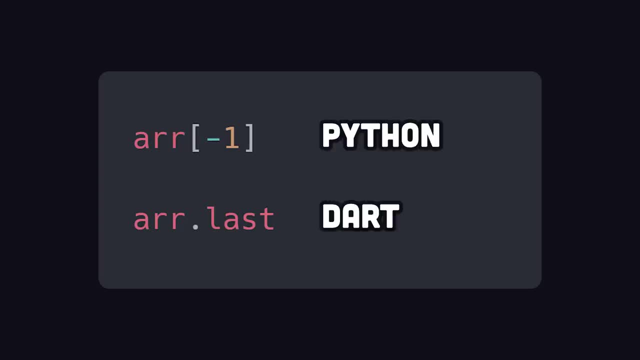 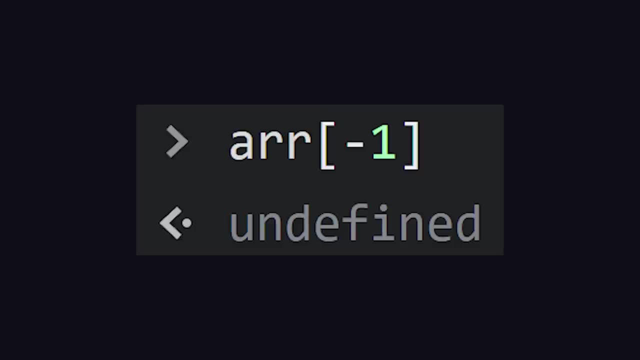 If you come from a language like Python, or most other languages for that matter, you might find it absurd that to get the last element in a JavaScript array you have to take the array length and subtract 1.. You can't just use negative 1 or last until now, because at makes this code obsolete. 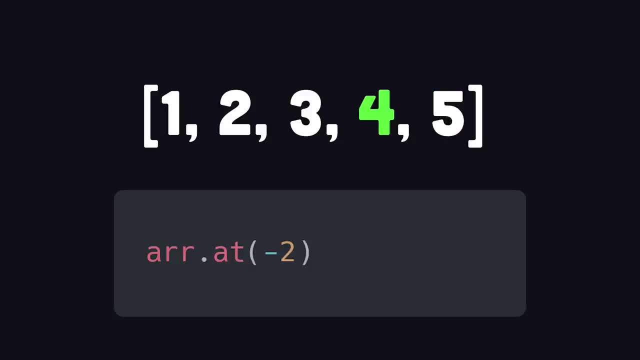 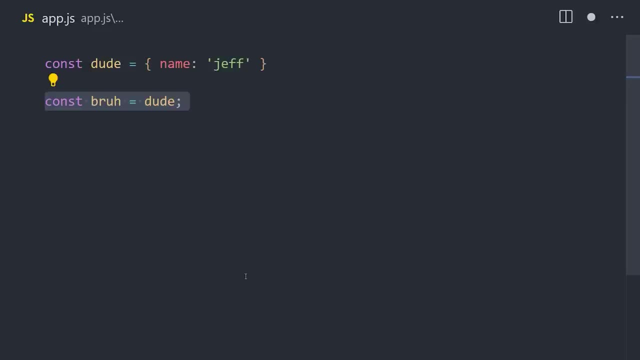 That's pretty cool, but deep copy is a little bit of a pain in the ass. That's pretty cool, but deep copy is a little bit of a pain in the ass. objects are passed by reference, which means if you assign one to a new variable, you're still. 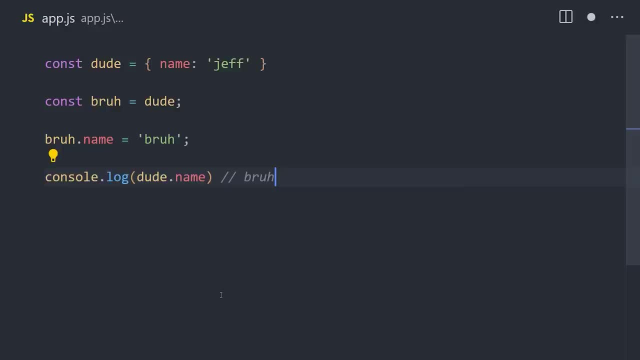 going to reference the same original object. If you modify a property on B, it will also modify the property on A because they're the same object reference. Now, most of the time we use object assign or the spread syntax to create a new object, but the problem here is that it only does a. 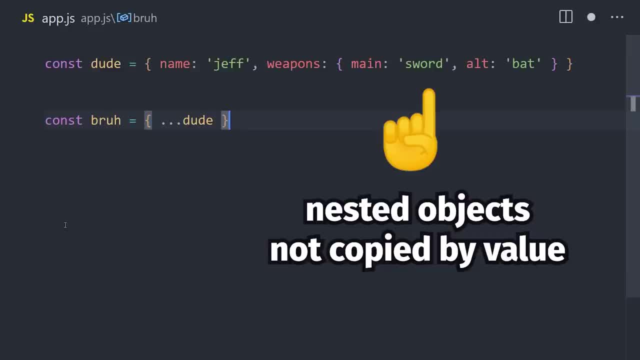 shallow copy, and that means if an object has any nested objects on it, those nested objects will still maintain the reference to their original object. But in many cases that's not what you want, and what developers have been doing for years is using JSON stringify to turn the object. 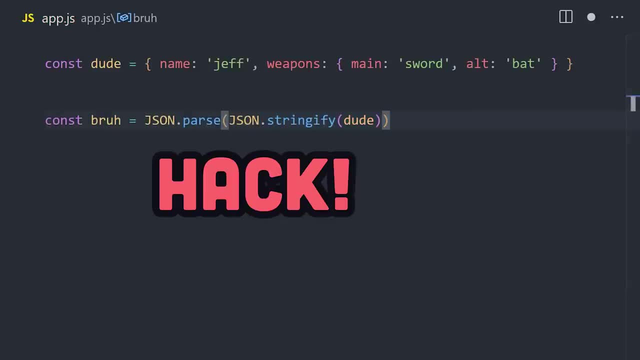 into a string and then JSON parse to parse it back into an object. That's a completely ridiculous hack that creates a new object reference in memory. but I'm happy to report that life doesn't have to be this way. There's now a global function called structured clone that can clone an object into